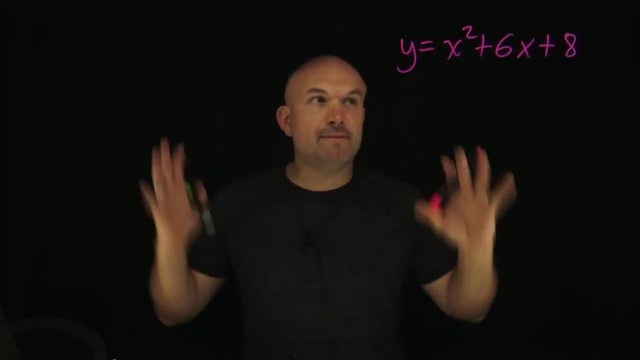 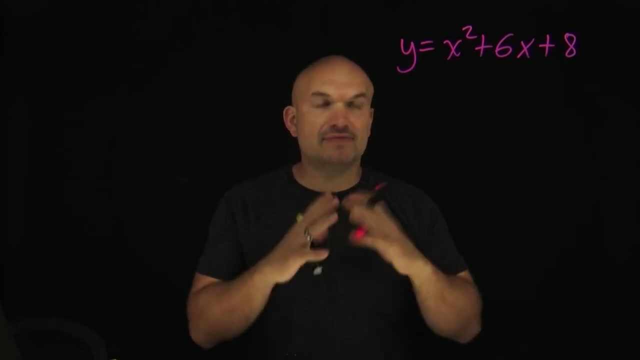 square to solve them. But in this example, what I want to do is just kind of like give you the basic idea of what we're trying to achieve when we are completing the square, And I think the main thing that I want you to understand is the idea of creating this perfect square. So let me just 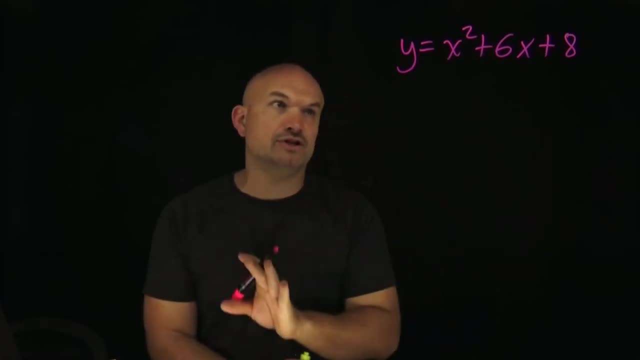 go ahead and change this out a little bit, and I think this is a rule that I want you to use anytime that you are struggling. One thing I always like to tell my students: like you know, when you're learning something, you're taking a test or anything else, and maybe the numbers kind. 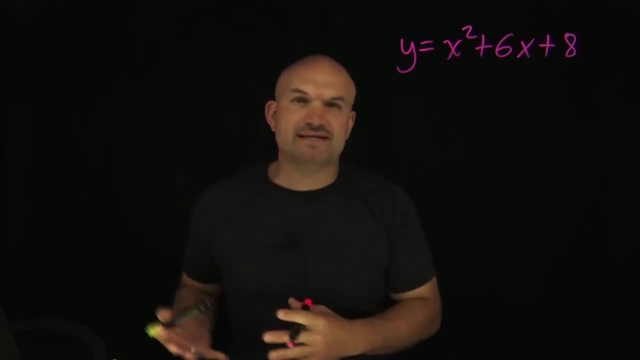 of seem tricky or you're not really sure what to do, like go back and use some basic numbers, okay, So what I'm going to do is I'm going to actually change this equation over here to something that's a little bit easier for me to understand. 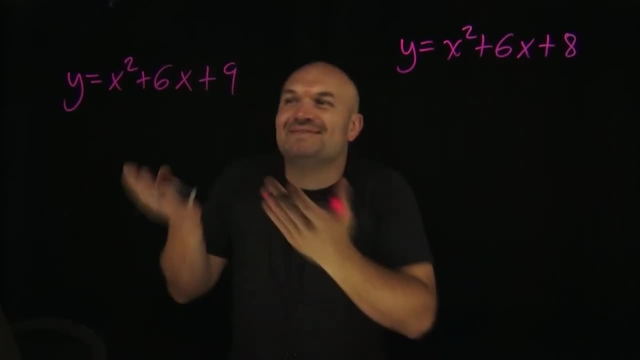 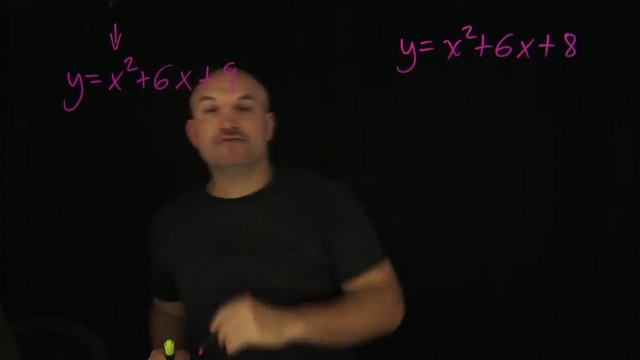 All right. now you might be wondering: well, why did you pick these numbers? like, what's special about this? Well, the reason. what's special about this is this is what we call a perfect square trinomial. Now, remember, perfect square trinomials are are going to be trinomials. that your first. 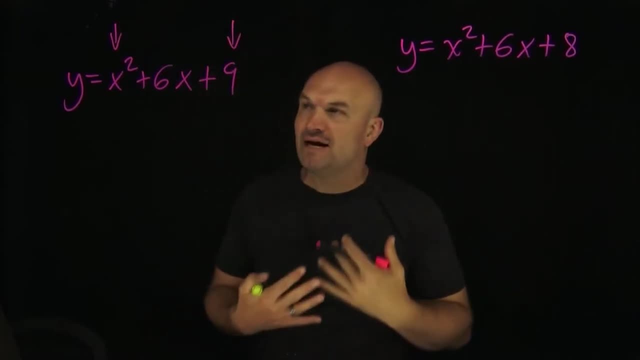 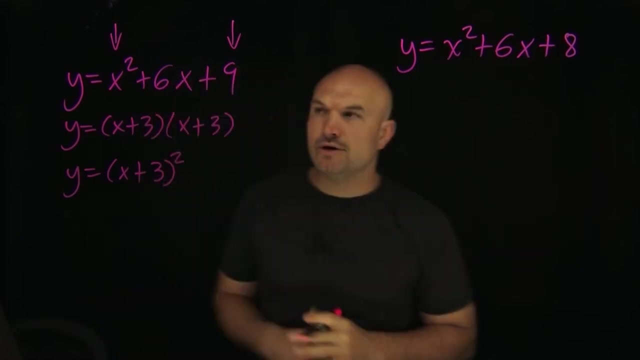 term are squared and your last term is squared, And what's so important about a perfect square trinomial is that they can be factored down into a binomial squared, So you can see, like in this example here, this is exactly what I'm looking for. 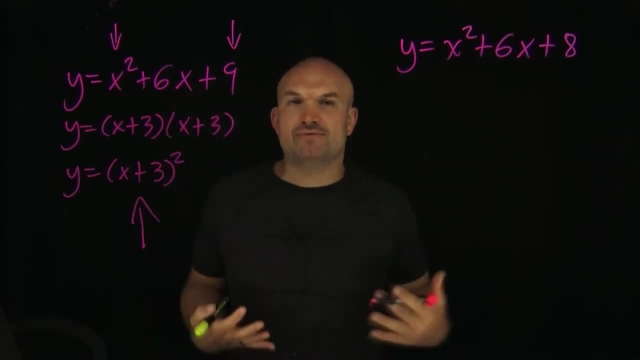 This is going to be my vertex form. That's what I'm trying to create when I am completing the square. One thing that I- you know, I want you to kind of idea is like when you're looking at, you know, trying to complete the square, I'm going to kind of go. 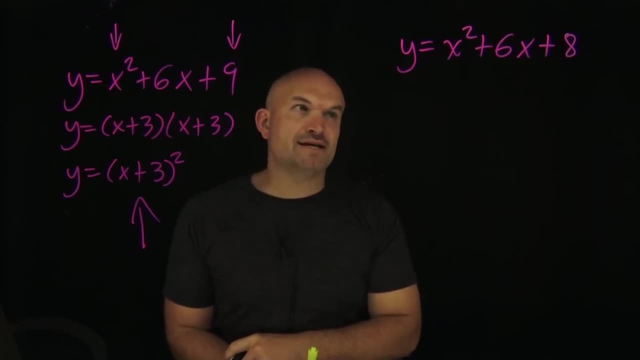 through this in two different methods, on two different ways. One thing I want you to think about is like: all right, if I need to take this and I need to create this binomial, squared right. that's what is putting things into vertex form Like: what number do I need? 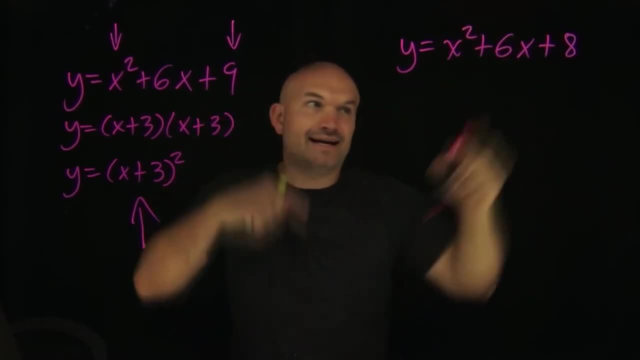 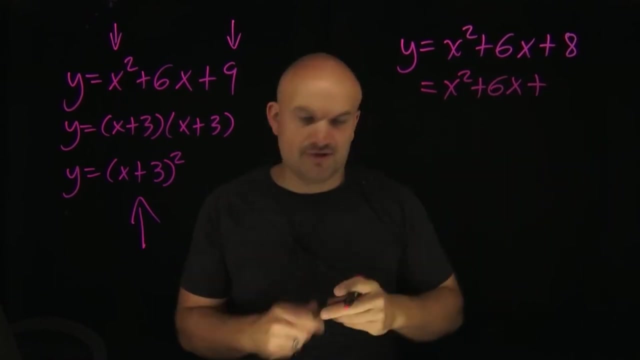 Well, obviously I already have an x squared and a six x, right, I just need that nine. I don't want the eight, I just needed that nine. So one thing you could do is just say: well, all right, well, why don't we just add the nine? then right, And let's just go ahead and add the nine. I'll make that in. 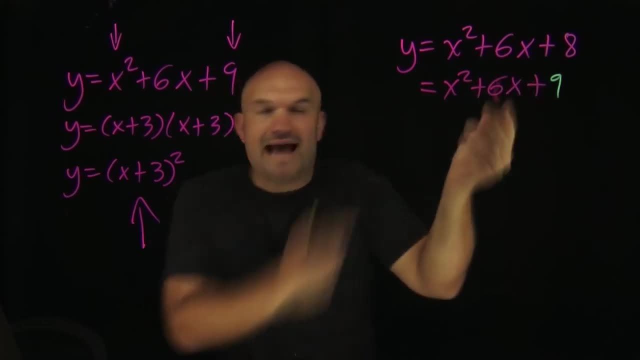 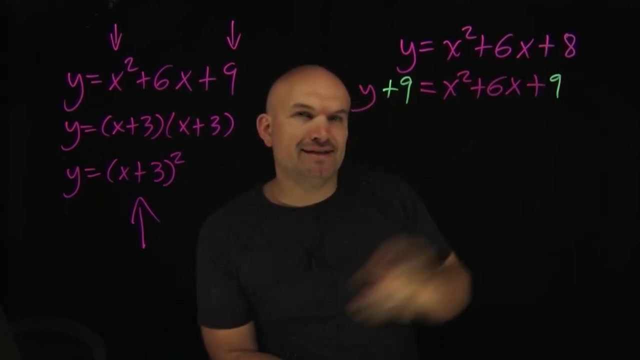 yellow here. And then obviously we know that well, you just can't like add a nine to one side, right? Remember, we like either going to add nine to one side, you have to add nine to the other side, All right. and then to remember, like the other thing is like, don't forget about the eight, Like 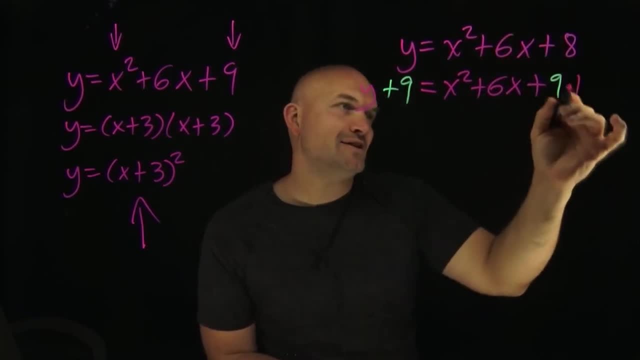 the eight's still there. I'm going to add nine to the other side. I'm going to add nine to the other side. You just can't like not forget about the eight, So let's just go ahead and write the eight over here. 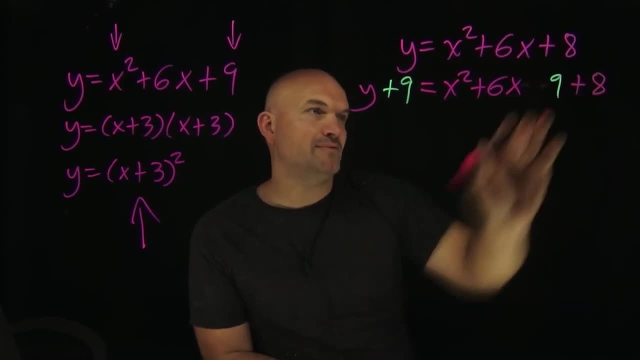 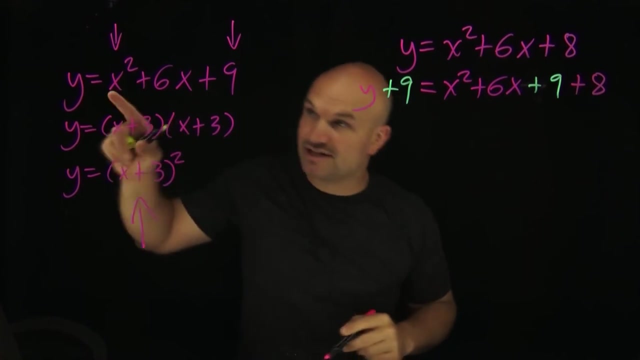 Okay, now here's something that's really important. Actually, let me write this in with there. Okay, so now what we did is we knew if we had an x squared plus a six x, we knew the number that was going to create that perfect square trinomial was a nine. So I just added that nine in there, right? 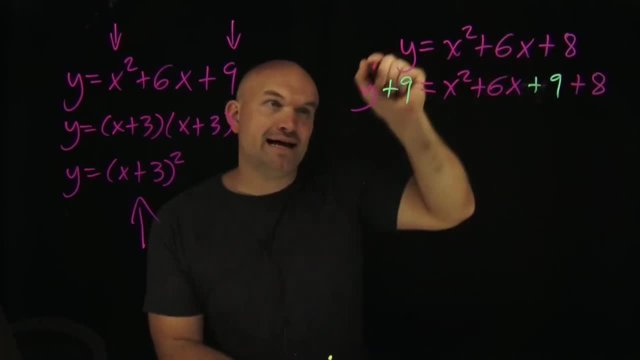 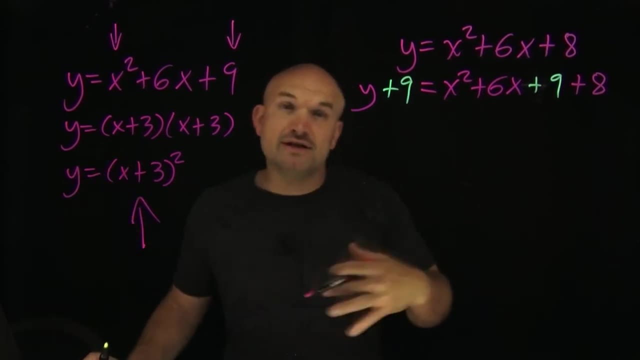 Kind of like some math magic, But it's okay, because I added a nine onto both sides, right? I mean again, if you have an equation, as long as you're doing one thing to one side, you're doing the same thing to the other side, it's going to be okay. You're still keeping an equivalent. 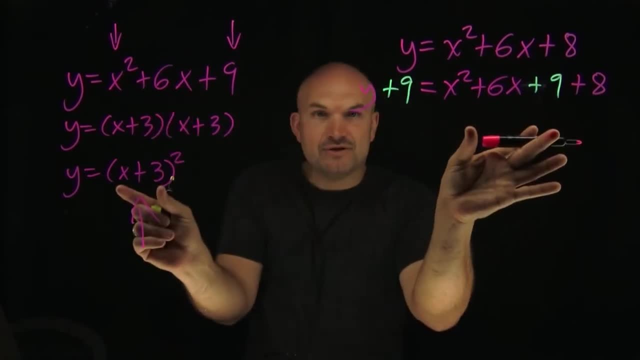 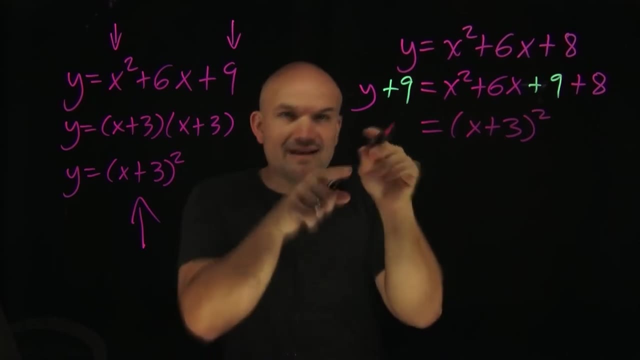 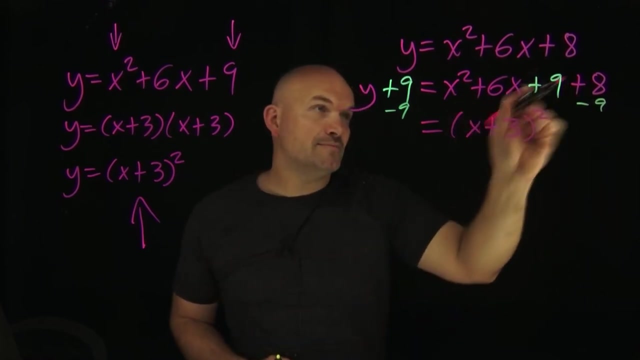 equation. So now I know that this factors down to this binomial squared. So now I can have a, let's say an x plus three quantity squared. Now again, if I want to solve for y, right, what are you going to do? Well, you're going to subtract a nine on both sides, and therefore remember this. 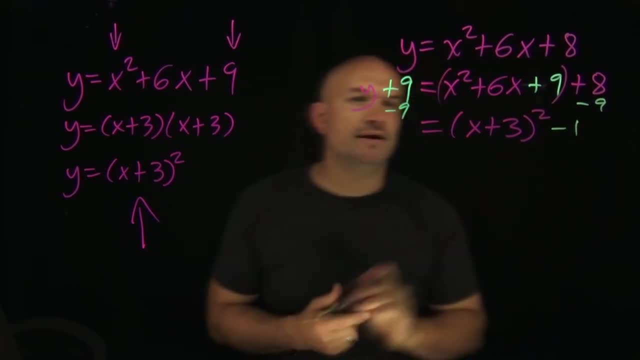 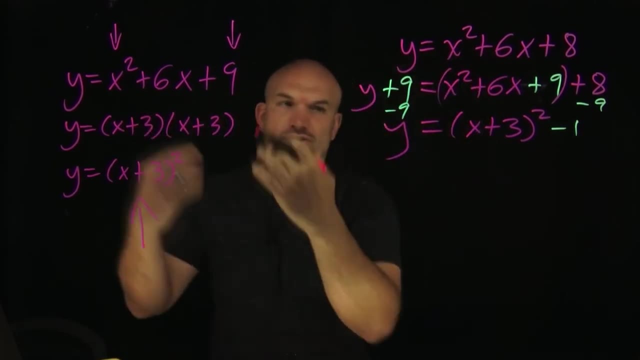 is going to there. So eight minus nine is going to be a minus one, and there you go. Now there is a way to kind of work through a problem when you kind of know what you're working with as far as creating a perfect square trinomial, 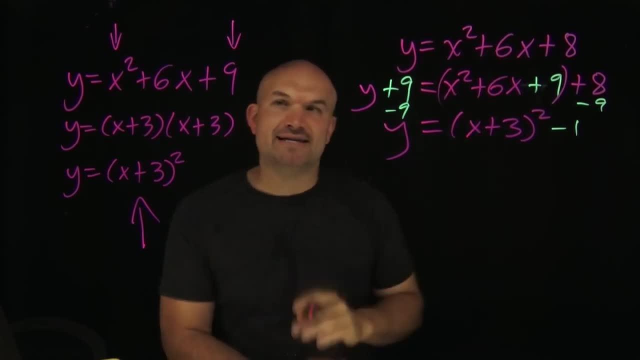 But let me go through this exact same process. if we didn't already recognize a perfect square trinomial, If we didn't know, x squared plus six x, that is going to give us nine. So let me just kind of do the exact same problem but also give you some different ways to kind of approach it. So 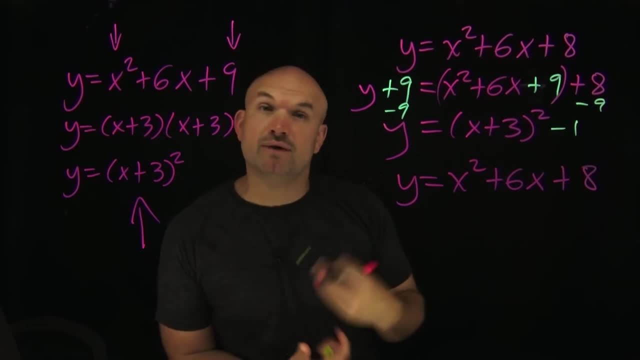 one thing that you always want to do is we have these first two terms. So, again, that is what you're going to want to look into: creating that perfect square trinomial. So what we'll do is we'll put parentheses around them. Then the next thing we want to do is, like: this one was obvious, right I? 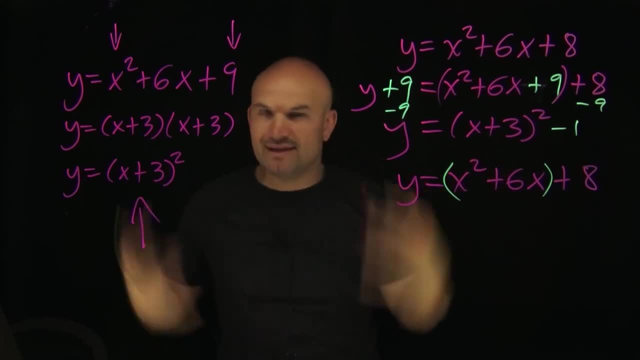 kind of like. I wanted you to recognize that relationship. But one of the hard things about completing the square is not always is it obvious that you're going to have a perfect square trinomial. Always is it obvious what the what, the value is that creates the perfect square trinomial? 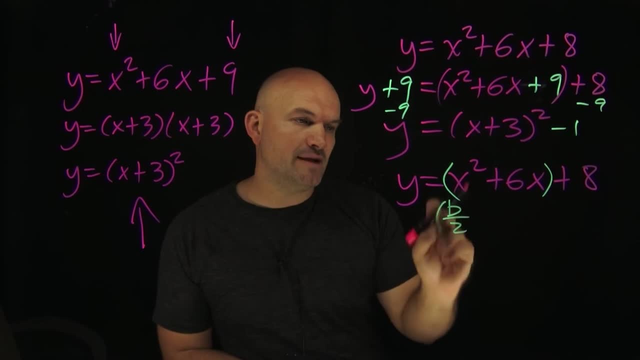 So what we can do to always find that value is: take our b divided by two and square it. So in this case, you would have a six divided by two squared, which is going to equal a nine. Now, rather than adding a nine to both sides, notice what I had to do. I just subtract it right from. 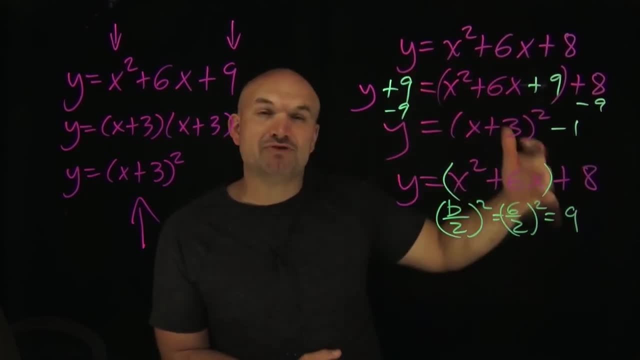 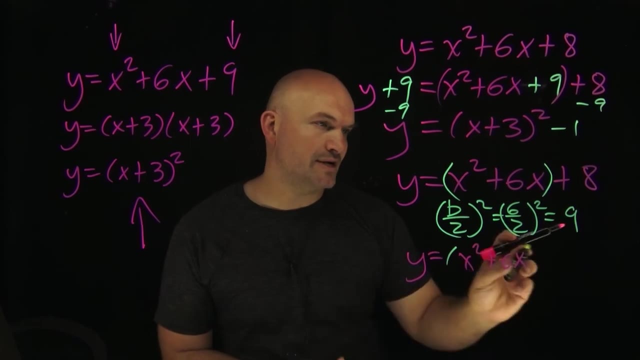 both sides to solve for the y. So what I like to do is I like to add and subtract it on the same side. So I have: y is equal to a x squared plus a six x. right? We're going to do a plus nine, and then we're gonna do: is a minus nine and then plus eight. right, because isn't that?